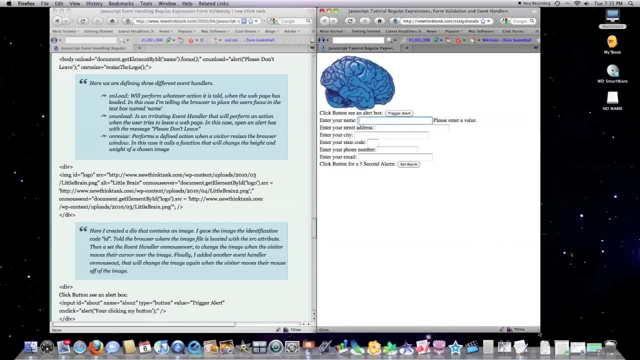 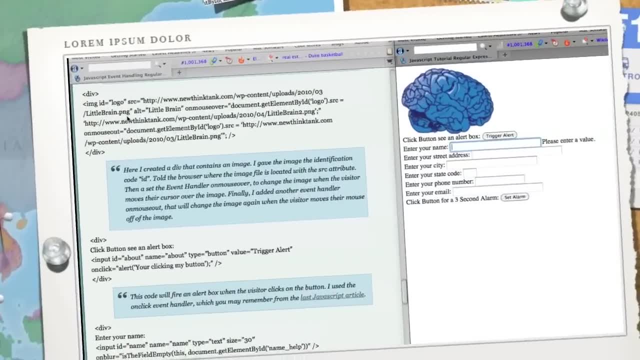 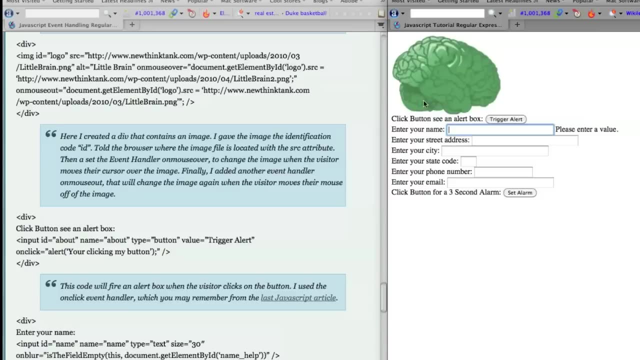 changes automatically. my image resets. There's a whole bunch of different things you can do with this, so that's another event handler. on resize. Now I also created a div and placed an image into it. You can see all kinds of event handlers are being triggered. I'm going to show you. 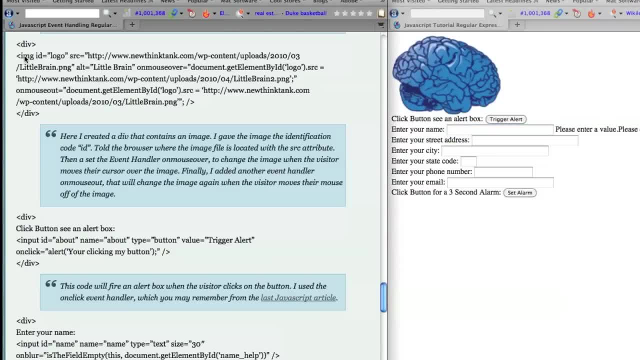 which ones those are. But first off, I created an image tag. I gave it an identification name logo in this example, and I said that the location of the image I want them to load when the web page loads up is this little blue brain right here, and this is where it's. 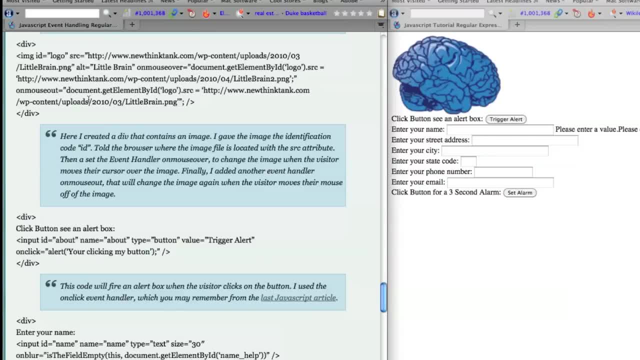 located Here's alt text. if you don't know what I'm talking about or this all looks foreign to you, watch my HTML tutorial. Then I used the on mouse over event handler and the document object and the function get element by ID and passed it the name of this image right here and said that I want to change the. 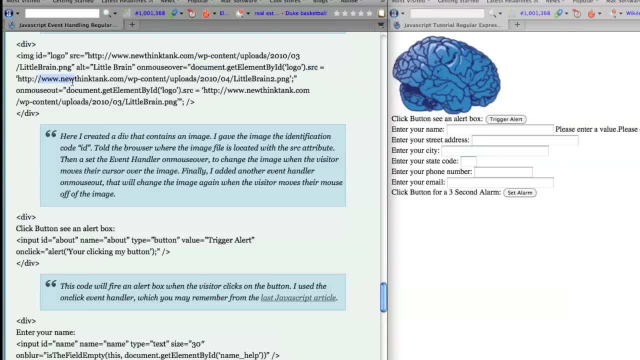 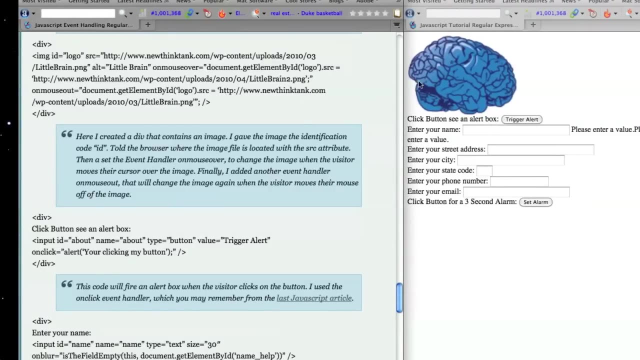 image source to this new image. and you can see here, if I roll my mouse over top of that image, it automatically changes. But why does it change back? Well, it changes back because I use the on mouse out event handler to call back the original image and place it right there. 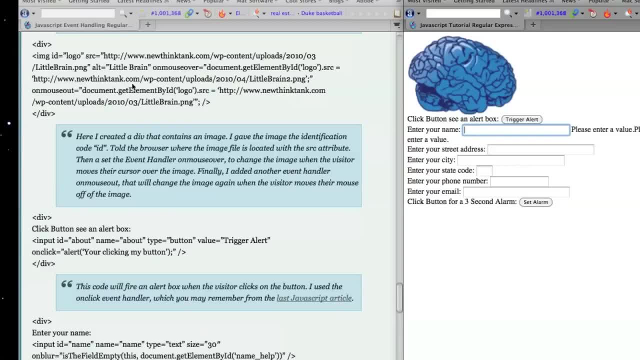 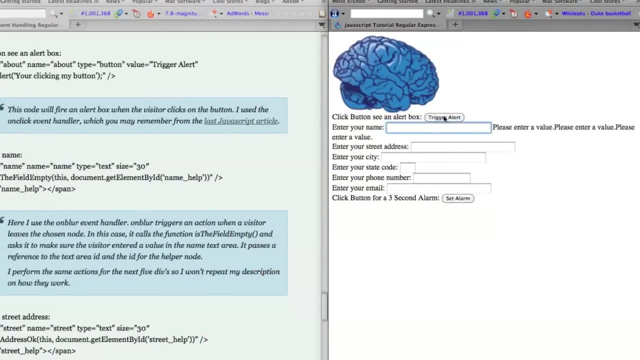 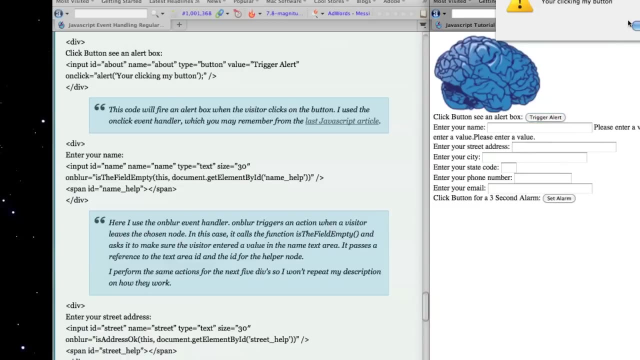 on the screen. So that's how you use, on mouse over and on mouse out, event handlers. Then I created another div area and put within it a button that's going to trigger certain actions. whenever this button is clicked, In this case, it's going to open an alert box, as you can see up here. So how did I do that? 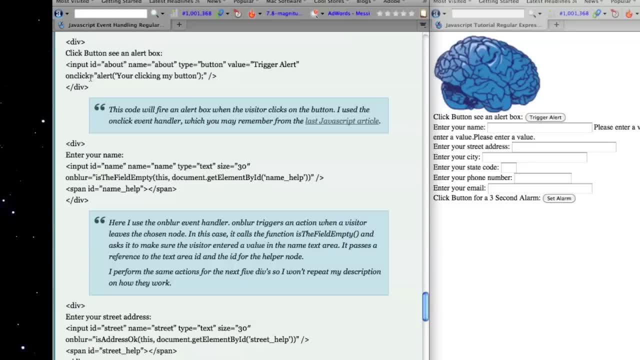 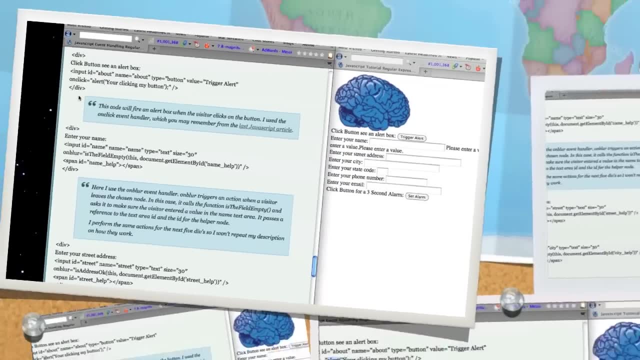 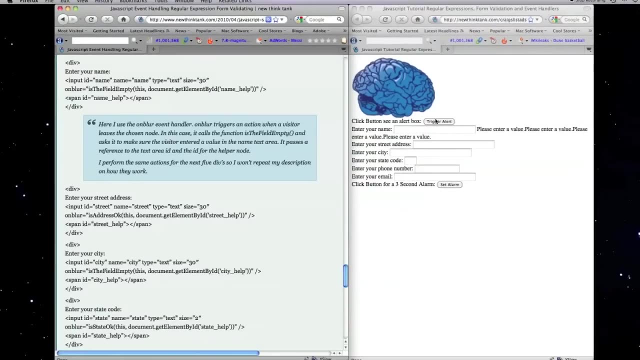 Well, I used an on click event handler, followed by, in double quotes, the calling of this alert function, which opens up an alert box on my screen, and then I close the div. Now is when we're going to start checking the text that people enter in to make sure that it's valid. I need to scroll out here. let's reload this window. 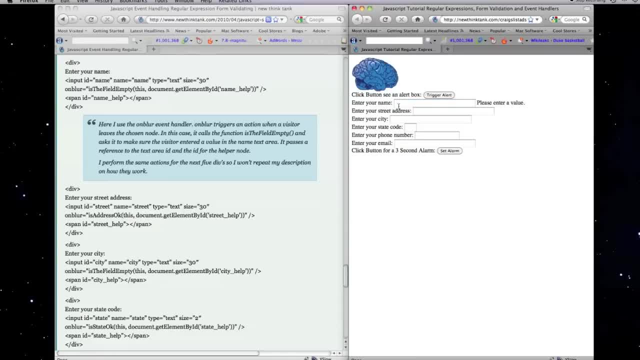 again. Now, if somebody- because the focus, remember, is set to this box- if somebody leaves that text area, you can see this value right here pop up. Let's do that again. See how it popped up. This is called your helper text. Well, what? 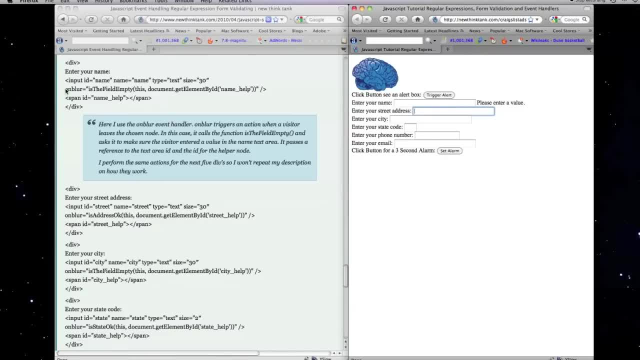 I'm doing in this field right here is I'm saying: when somebody leaves the text box, let's do it again. you can see that helper text popped up there. When somebody leaves that text box area, I want the on blur event handler to occur and the on. 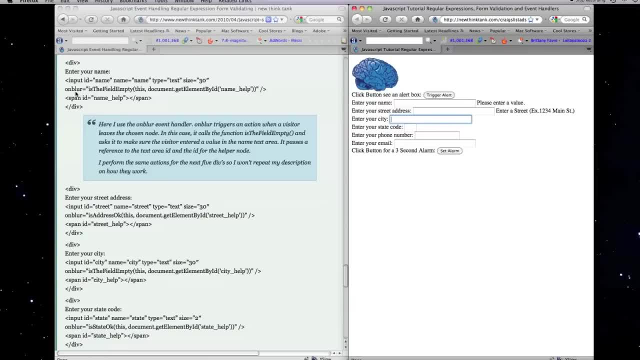 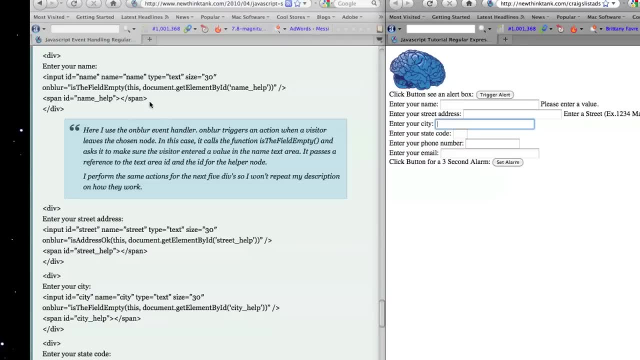 blur means leaving text area, just like you saw right there, And whenever somebody leaves that text area, it's going to call this function right here, which is the onblur, is the field empty function, and it's going to pass the identification number for this text. 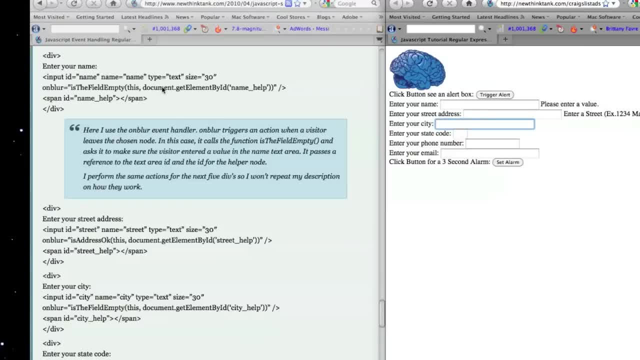 that's either entered or not entered, and then it's going to pass an identification name for the helper text using the document object, followed by the get element by id function, just like before, and then I create a span inside of the div and I give it the name name, underscore help. so that's. 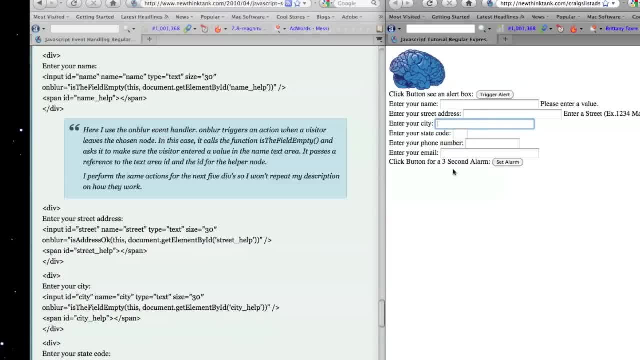 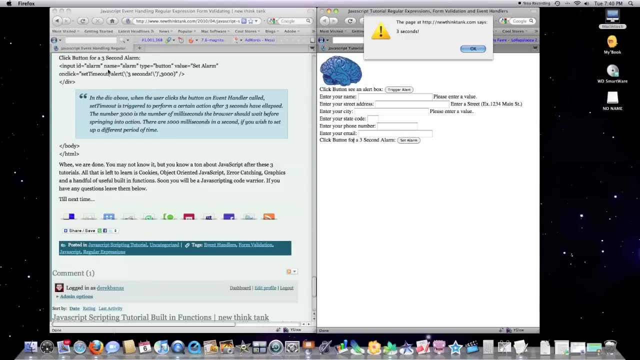 what that div does, and that also is what all of these other divs do, except for this. down here I have, I have set an alarm button in which, when somebody presses that alarm after a certain period of time, an alert box will open and you can see the code right here for this event. I again 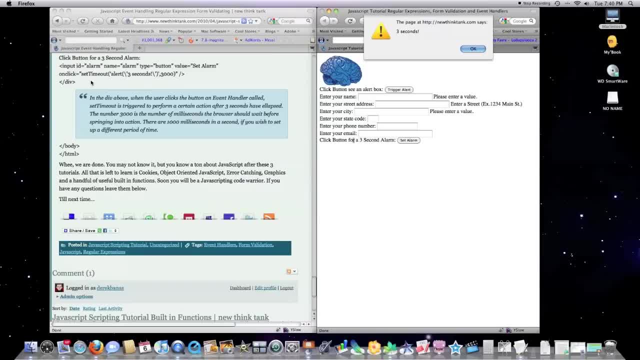 trigger an on click of the button element. that's there. and then I said, whenever the mouse is clicked, I want you to wait a certain period of time, in this case three thousand milliseconds or three seconds, and I want you to open alert box that states three seconds in it. you can see that. all right, there again the function you call to trigger an event. 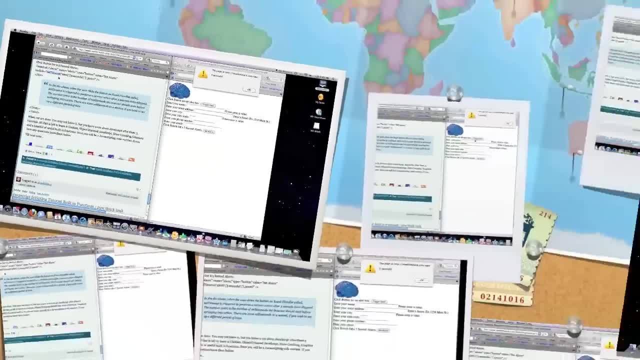 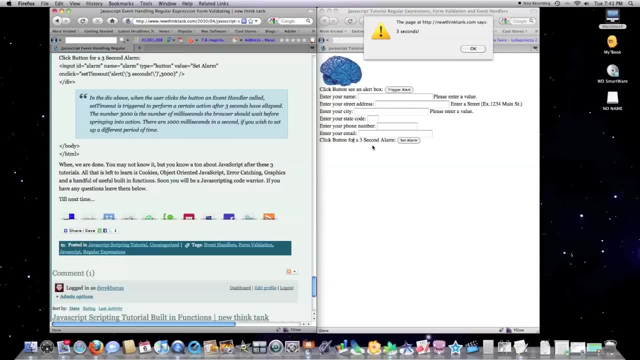 after a certain period of time is the set time out, and that is basically everything that this web page does. however, I don't have the time to go through all of the functions that this little guy here calls, but I will in the next tutorial, and then I'll also teach you about a.